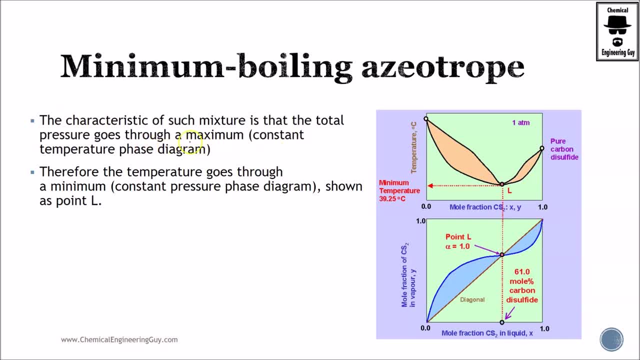 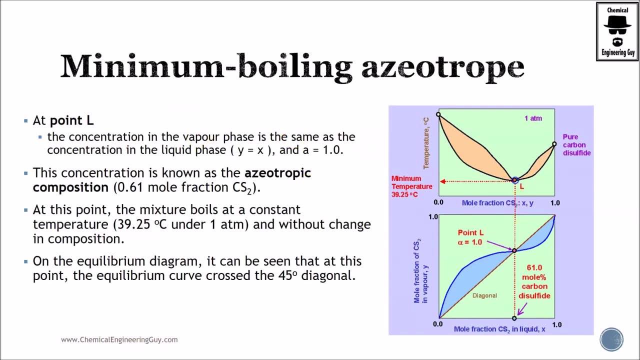 Okay. so what do we have here? Okay, I said it before: minimum boiling azootrope will have a maximum point whenever we have constant temperature, and we will have a minimum point when we have a constant pressure. Now here is the point I was telling you about. let's call point L. At this point, we have a solution. 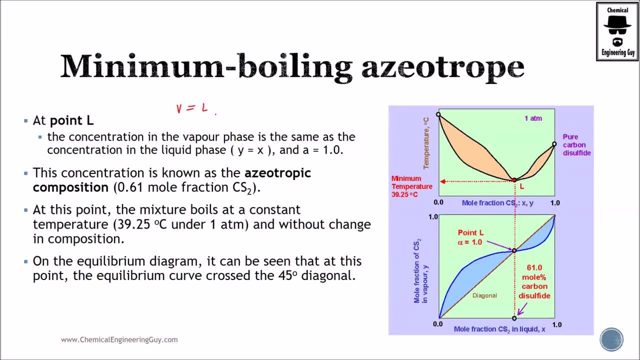 or a vapor that has the same compositions as the liquid. So technically, there is no vapor liquid mixture. even though there is, is actually a a point. so remember, whenever you have crossing lines, especially in functions, the point is a single point doesn't mean that you have area. so that's why, technically speaking, 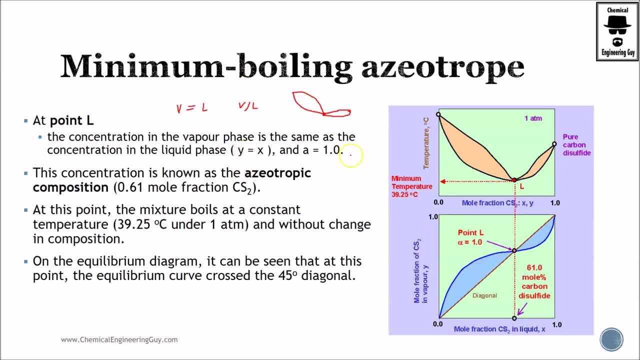 you could say that there is no vapor liquid phase. and what is true? y equals x, so y a will be equal to x a, meaning that the composition in the liquid and vapor phases are the same. and if that is true, the driving force will not be enough to carry out this separation via desolation. 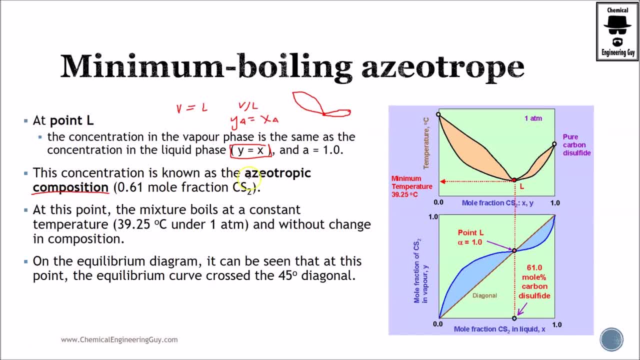 this concentration is known as the azeotropic composition. yeah, very creative. what is the composition in the azeotrope? yeah, the composition is found here. at this point, the mixture boils at the constant temperature. that's also very important. we will not be able to change. 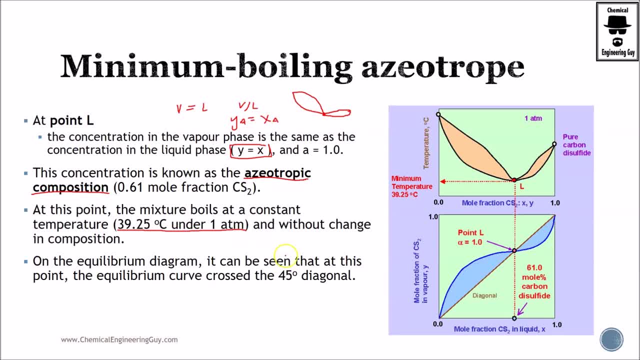 that the only thing that we can do is either pressurize it or add another uh external ingredient to favor the change or shift of the azeotrope. on the equilibrium diagram, it can be seen that at this point we have the line with the 45 degrees. yes, so this is temperature versus. 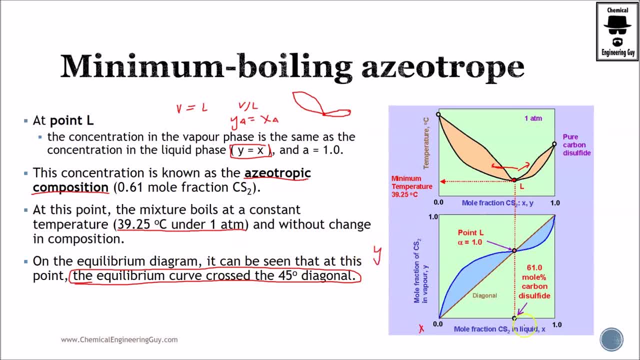 composition. but let's go to composition versus uh, liquid composition and vapor composition. remember that if we have a crossing in the x? y diagram or the 45 degree line, then we will know that we will not be able to carry out our desolation. now we know that this is the azeotropic point.